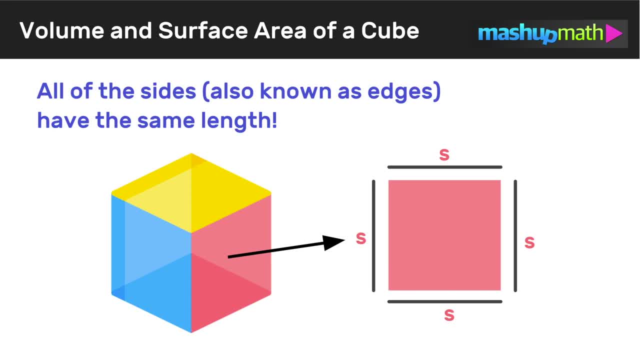 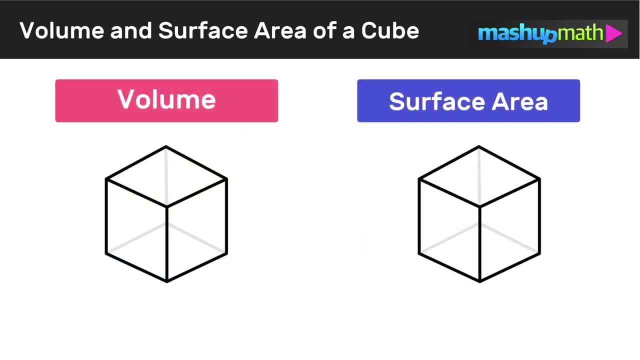 all of the sides, also known as edges, have the same length. So in this case we're going to call that length s, And now we are ready to explore the difference between the volume of a cube and the surface area of a cube. So let's 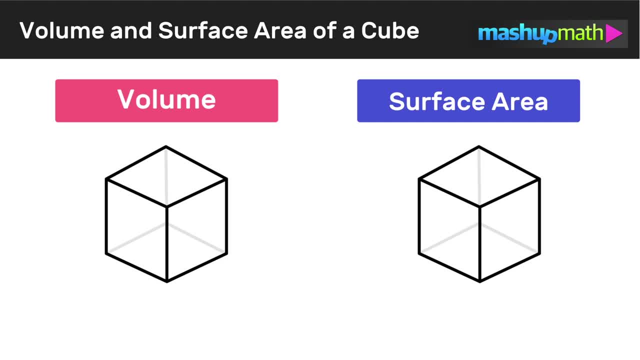 start with the volume of a cube. The volume of a cube is the number of cubes it would take to completely fill the inside of the figure. So we can think of volume as the total number of unit cubes it would take to completely fill up the inside of a cube. 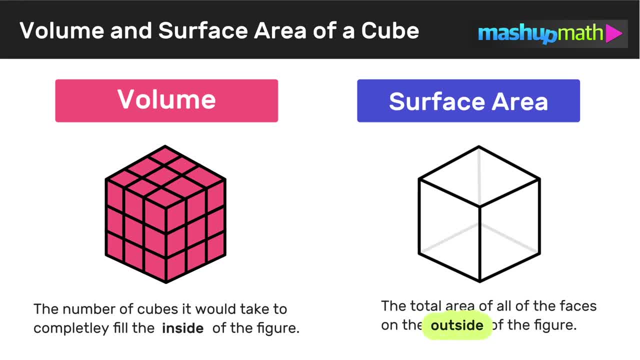 The surface area of a cube is the total area of all of the faces on the outside of the figure. So volume was inside, surface area is outside And we can think of surface area like all of the space we would need to paint on the outside of a 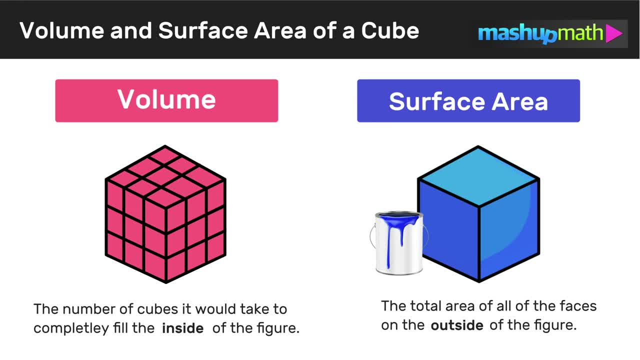 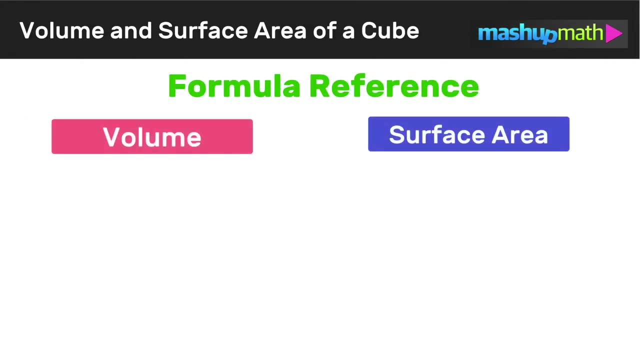 cube if we wanted to paint it completely one color. So now that we understand the difference between volume and surface area, let's go ahead and look at some formulas that we can use to solve problems. And now we are ready to take a look at the formulas for finding the. 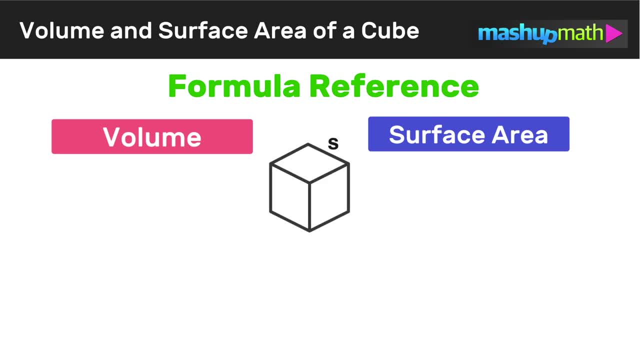 volume and surface area of a cube. So when we have a cube with side length s, the volume is equal to the sides cubed or s to the third power. And remember that volume is measured in cubic units. And for surface area, surface area is equal to 6 times s squared, so 6 times the 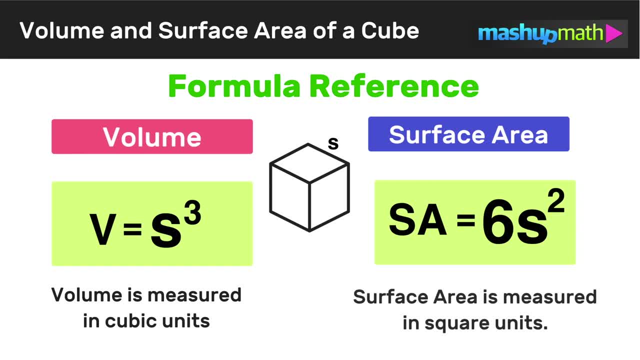 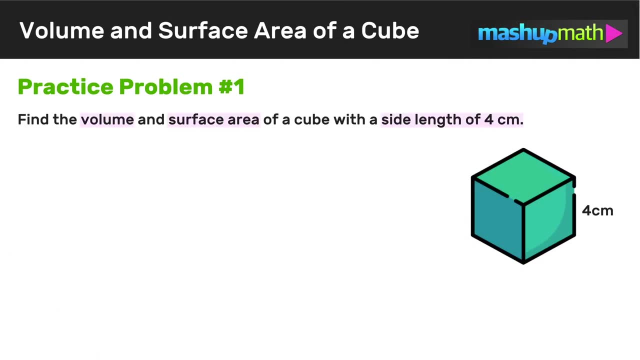 length of the side squared, And remember that surface area is measured in square units. So let's keep these formulas in mind as we go ahead and work through a few practice problems. Alright, so here's our first example where we have to find the volume and 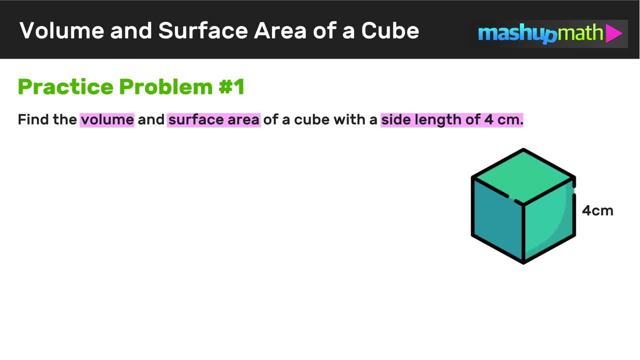 surface area of a cube with a side length of 4 centimeters. So in this example, our value for s is just 4, since every side length of this cube equals 4.. Now to find the volume and surface area of this cube, we are going to use our formulas. So let's start off. 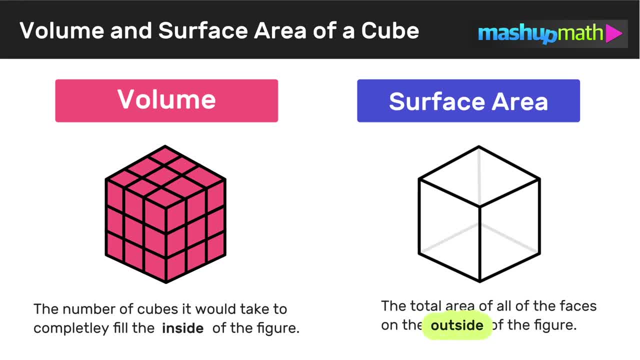 The surface area of a cube is the total area of all of the faces on the outside of the figure. So volume was inside, surface area is outside And we can think of surface area like all of the space we would need to paint on the outside of a 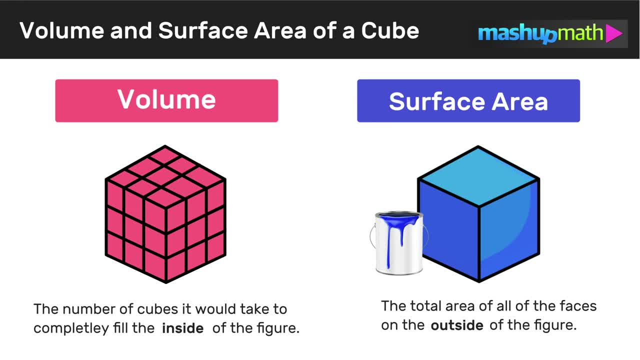 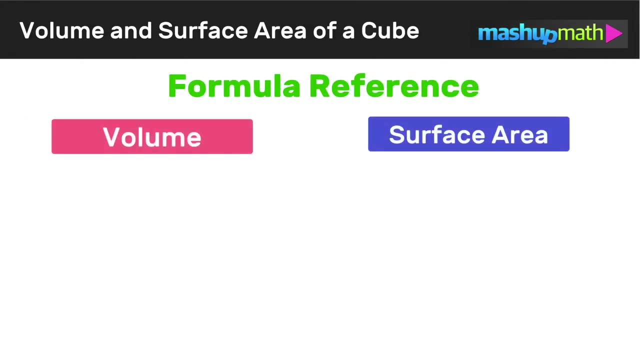 cube if we wanted to paint it completely one color. So now that we understand the difference between volume and surface area, let's go ahead and look at some formulas that we can use to solve problems. And now we are ready to take a look at the formulas for finding the. 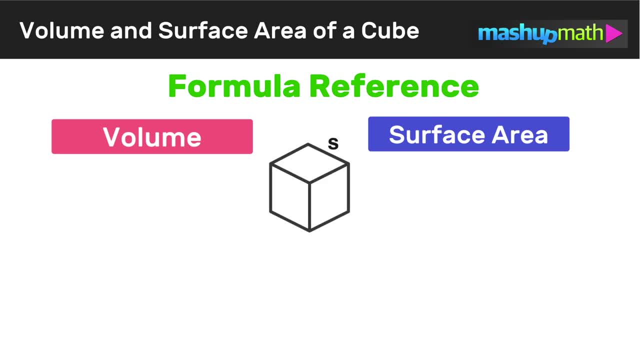 volume and surface area of a cube. So when we have a cube with side length s, the volume is equal to the sides cubed or s to the third power. And remember that volume is measured in cubic units. And for surface area, surface area is equal to 6 times s squared, so 6 times the 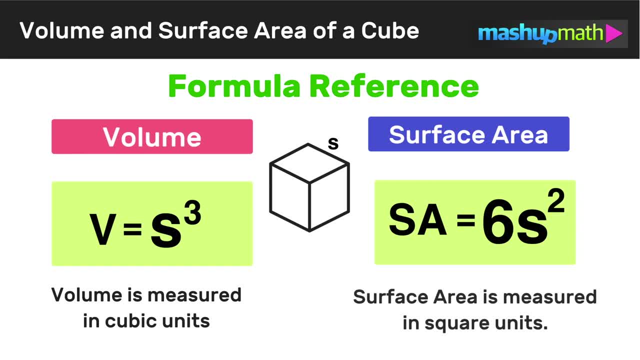 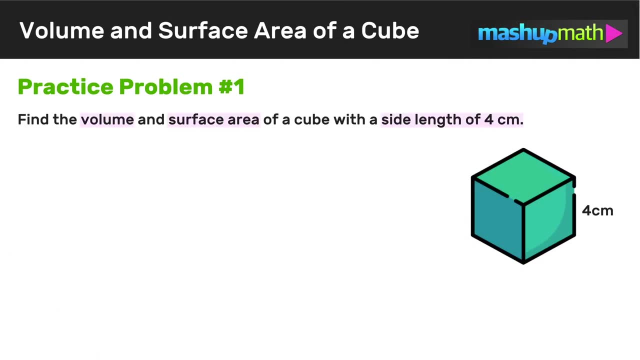 length of the side squared, And remember that surface area is measured in square units. So let's keep these formulas in mind as we go ahead and work through a few practice problems. Alright, so here's our first example where we have to find the volume and 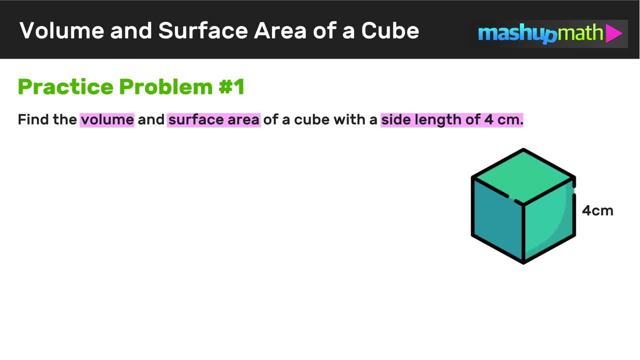 surface area of a cube with a side length of 4 centimeters. So in this example, our value for s is just 4, since every side length of this cube equals 4.. Now to find the volume and surface area of this cube, we are going to use our formulas. So let's start off. 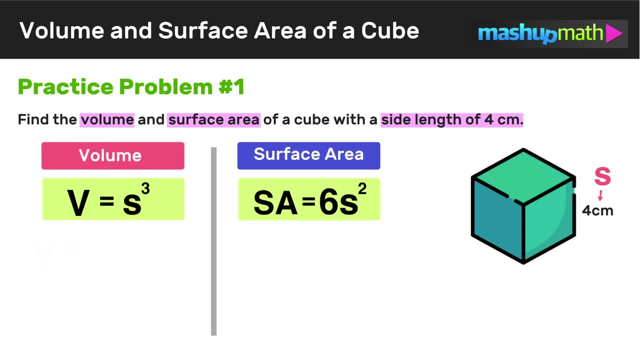 with volume. Again, the volume formula is that v equals s cubed. So in this case v equals 4 cubed. 4 cubed is equal to 4 times 4 times 4, which we know is equal to 64. And so the 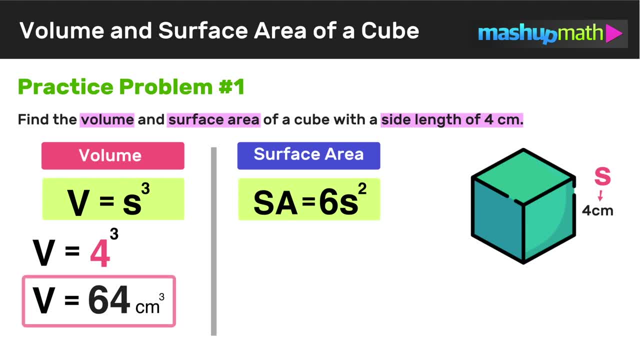 volume of this cube is 64 cubic centimeters. The next thing that we have to do is find the surface area, And again we're going to use a formula. The surface area formula says that surface area equals 6 times s squared, or 6s squared. 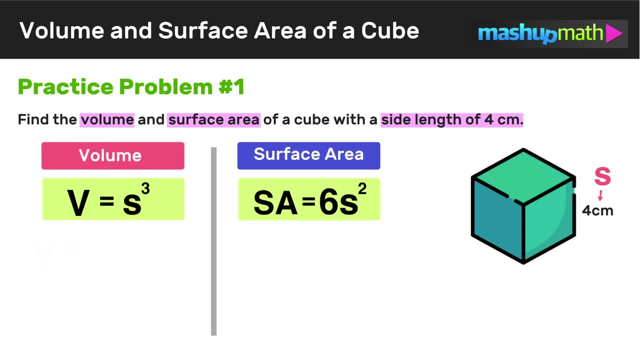 with volume. Again, the volume formula is that v equals s cubed. So in this case v equals 4 cubed. 4 cubed is equal to 4 times 4 times 4, which we know is equal to 64. And so the 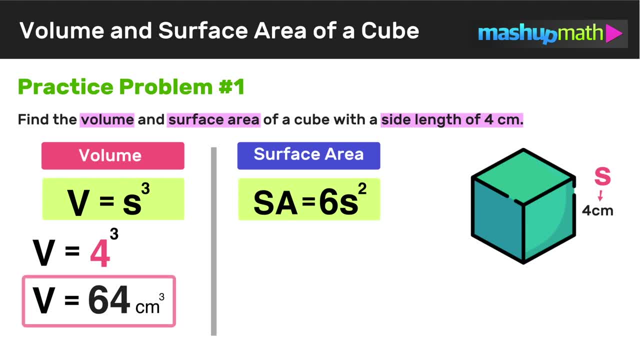 volume of this cube is 64 cubic centimeters. The next thing that we have to do is find the surface area, And again we're going to use a formula. The surface area formula says that surface area equals 6 times s squared, or 6s squared. 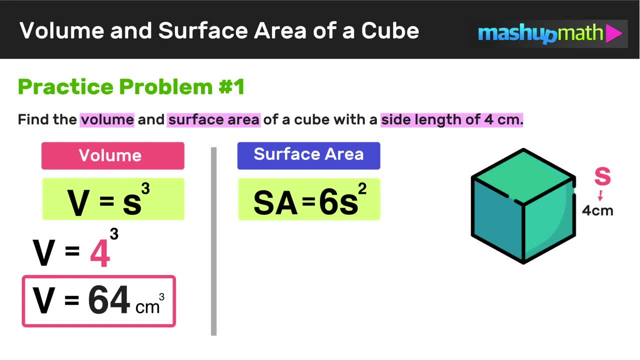 where s is equal to the side length of the cube. In this example it is 4.. So instead of 6 times s squared, we have 6 times 4 squared, And now we can just work this out: 6 times 4 squared. we know that 4 squared is equal to 16.. So the surface 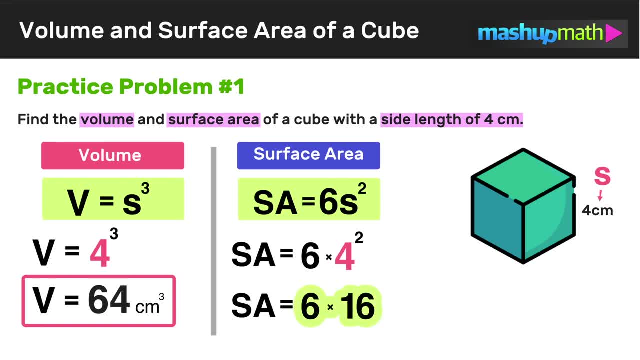 area equals 6 times 16, which is equal to 96.. So the surface area of this cube is 96 centimeters squared. So in future examples the value for s will always be different, but the formulas will always stay the same. 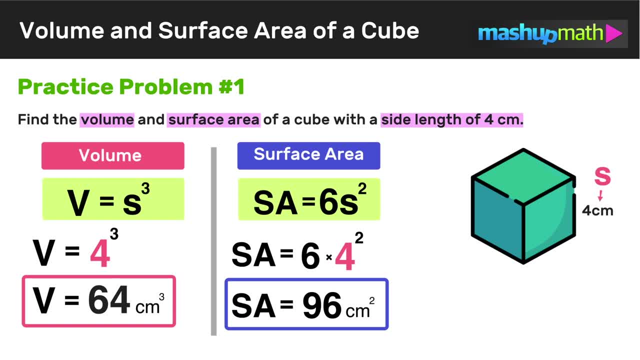 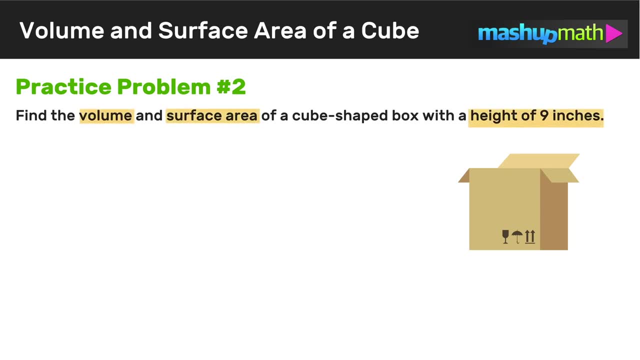 As long as you understand how to apply the formulas, you'll be able to solve problems involving finding the volume and surface area of a cube. Let's go ahead and take a look at one more example. In this second example, we have to find the volume and surface area of a cube-shaped box with a height of 9 inches. 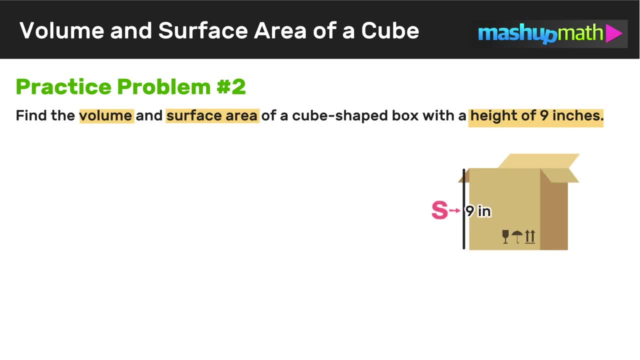 Since we are dealing with a cube in this problem, we know that all of the side lengths will be equal to 9.. So in this example, our value for S is 9.. And now we are ready to go ahead and use that value for S in the volume and surface area. 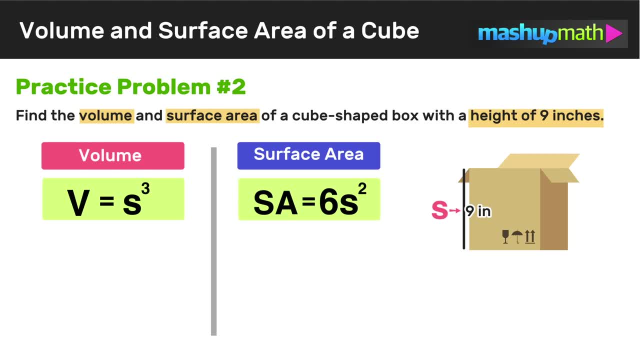 of a cube formulas and we can solve this problem. So let's start off with volume. Volume equals S to the third power, in this case 9 to the third power. We know that 9 times 9 times 9 is equal to 729, and we can conclude that the volume of 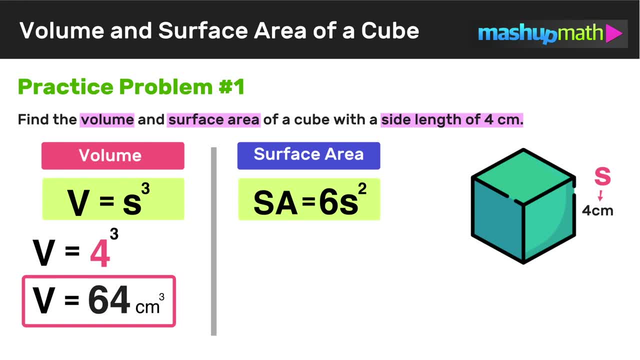 where s is equal to the side length of the cube. In this example it is 4.. So instead of 6 times s squared, we have 6 times 4 squared, And now we can just work this out: 6 times 4 squared. We know that 4 squared is equal to 16.. So the 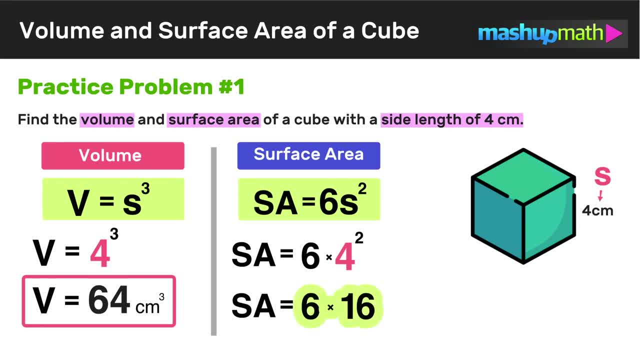 surface area equals 6 times 16,, which is equal to 96.. So the surface area of this cube is 96 centimeters squared. So in future examples the value for s will always be different, but the formulas will always stay the same. 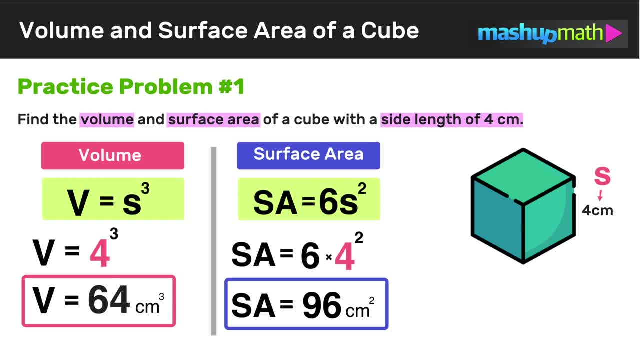 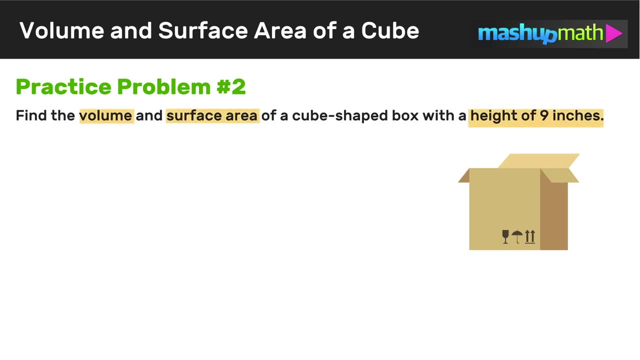 As long as you understand how to apply the formulas, you'll be able to solve problems involving finding the volume and surface area of a cube. So let's go ahead and take a look at one more example. In this second example we have to the volume and surface area of a cube shaped box with a height of 9 inches. 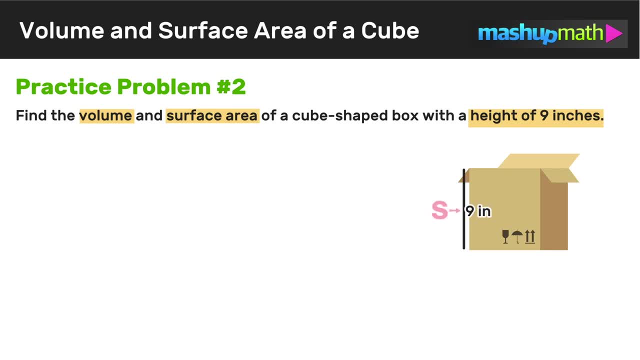 Since we are dealing with a cube in this problem, we know that all of the side lengths will be equal to 9.. So in this example, our value for S is 9.. And now we are ready to go ahead and use that value for S in the volume and surface area of. 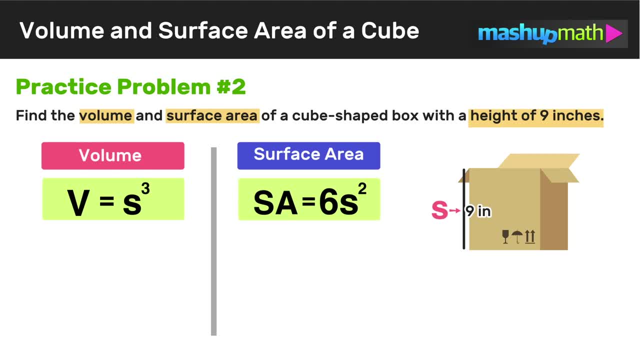 a cube formulas and we can solve this problem. So let's start off with volume. volume equals S to the third power, in this case 9 to the third power. We know that 9 times 9 times 9 is equal to 729 and we can conclude that the volume of 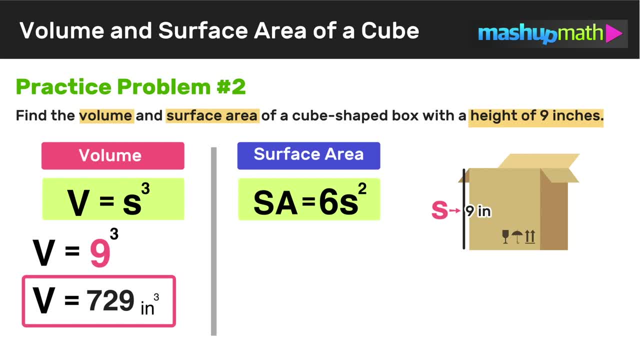 the box is equal to 729 cubic inches. Now the last thing that we have to do is find the surface area of the box, and we know that surface area equals 729.. 6s squared- In this case s again- is equal to 9, so surface area equals 6 times 9 squared. 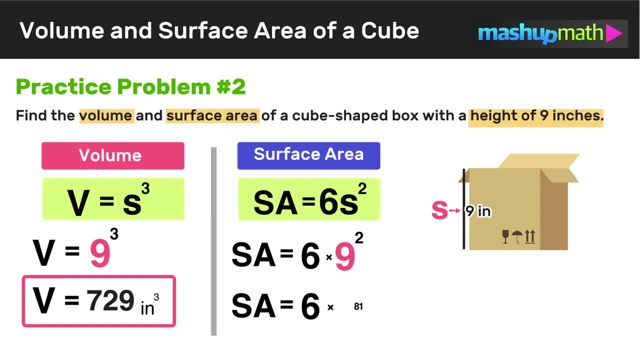 So we know that 9 squared is equal to 81,, so the surface area is equal to 6 times 81, and 6 times 81 is equal to 486, and we can conclude that the surface area of the box is equal to 486 square inches, And that's all there really is to it when it comes to finding. 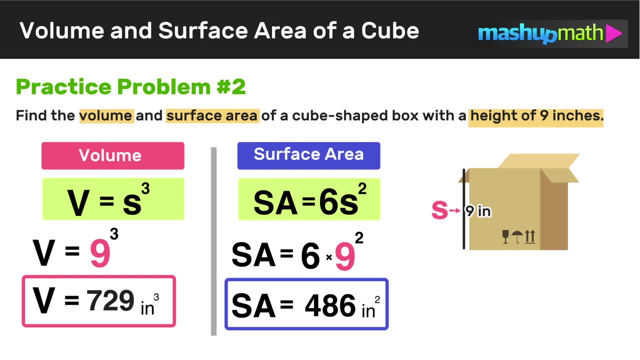 the volume and surface area of a cube. If you understand the formulas, it's pretty straightforward. So now I'm going to leave you with one more practice problem that you can try on your own, just to practice a little bit more, and I'll see you guys all soon. 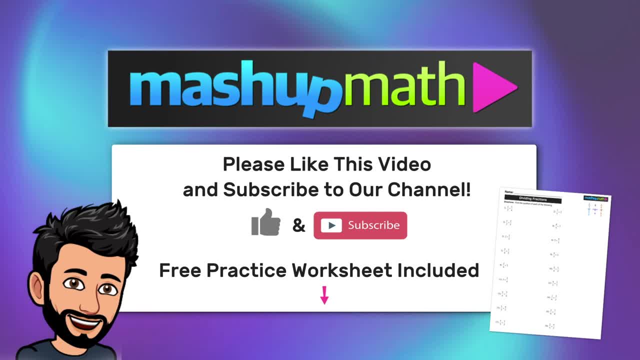 Hi everyone. Anthony here one last time. Hope you found that lesson to be helpful And if you want to help us out, please like the video and subscribe to our channel. We're committed to adding new video lessons every week and now would be the time to subscribe. 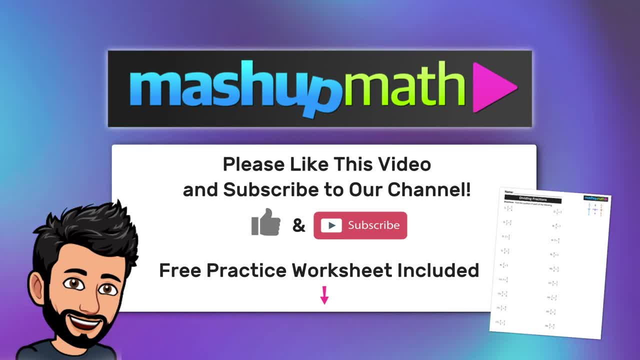 so I really hope that you will consider it And also don't miss your chance to download your free practice worksheet that's included with this video lesson. Just click the link in the description below and you can get your download. Hope to see you all soon. Bye. Thanks for watching.